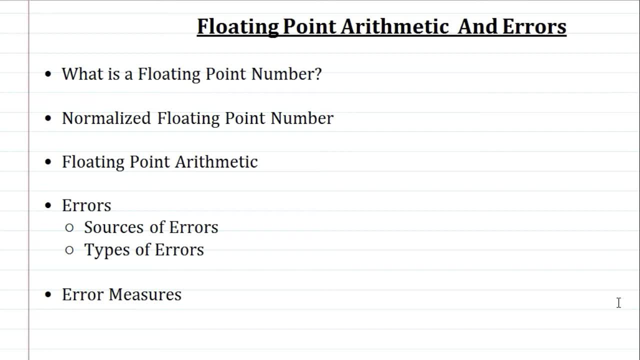 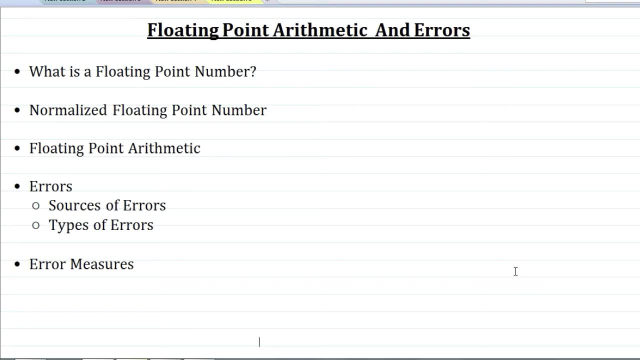 and then we will be learning what is a normalized floating point number, how to do arithmetical operations or floating point numbers that is addition, subtraction, how to do that. So there are certain basic laws of arithmetic that we will be covering here, and then what all errors are possible. 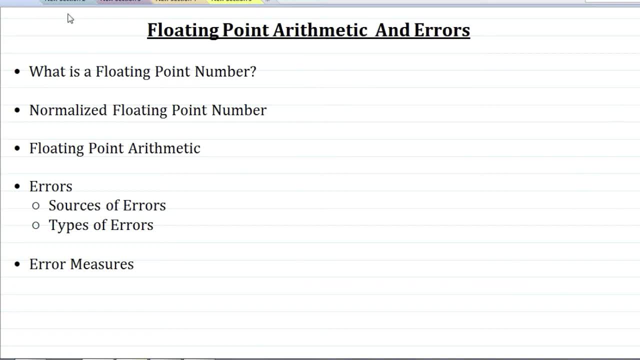 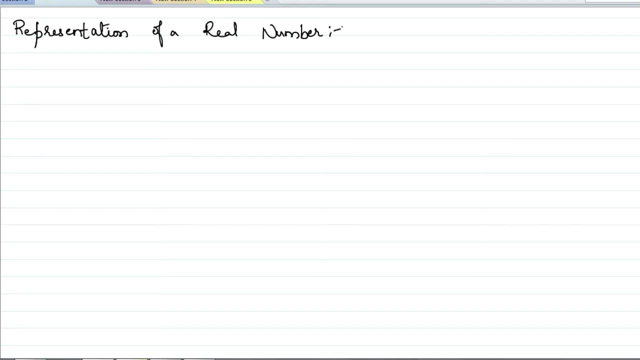 what are the sources of errors, types of errors and various formulas for measuring. what is the errors that has occurred in your solution? The first topic, what we will be learning here, is representation of a real number. There are two ways of representing a real number. 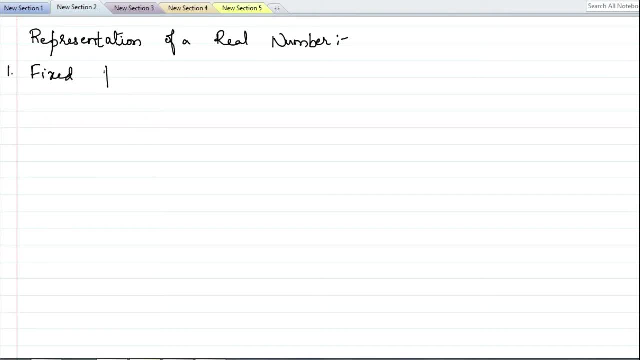 So one is the fixed point representation and the other one is a floating point representation. So what is fixed point representation? As the name suggests, fixed point representation is where the decimal point is fixed in the number. Example is 12.56.. 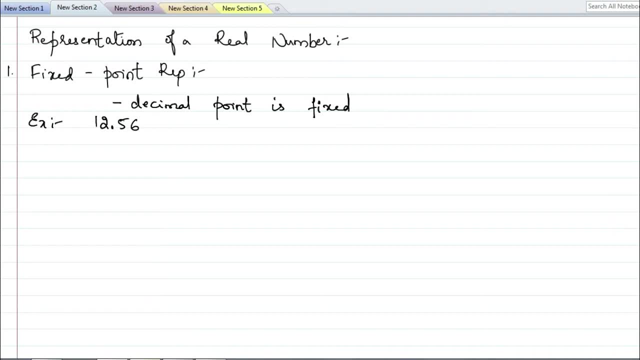 So here this is one simple example wherein the decimal point is fixed. So this type of representation, So this type of representation of numbers is called as fixed point representation. This is the type of representation we use in our day to day calculations. 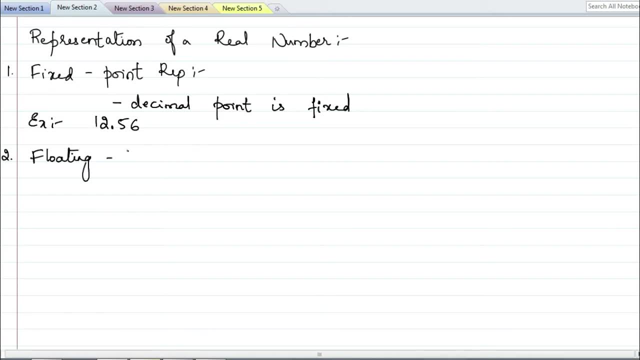 Now the next representation is floating point representation. In this representation the decimal point will be floating. It means the point moves to and fro depending on the value of the exponent in the given number. So let us take the same number, 12.56.. 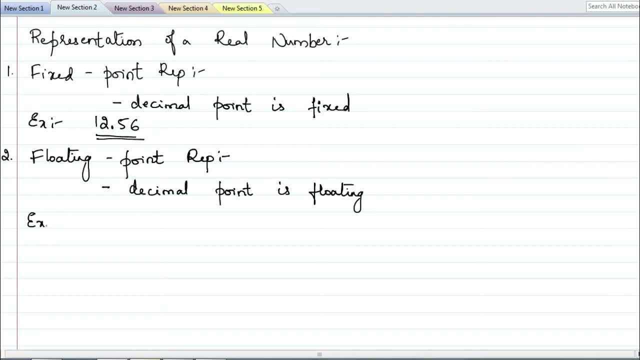 This 12.56 can be written in various forms, So I will write some of the forms here. The value remains same, but we will see various representations of this number. Say, the same number can be written as 0.1256 into 10 square. 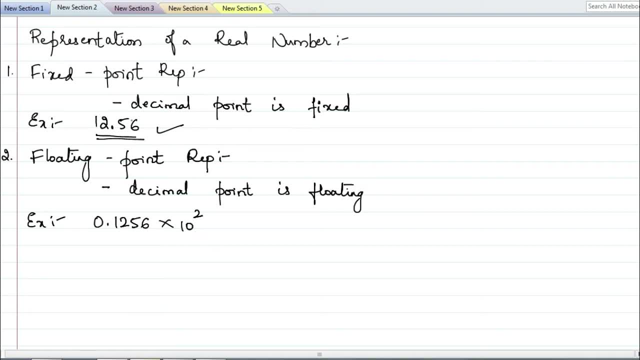 Now simplify this number: 0.1256 into 10 square is 100.. When you multiply 100, you will get 12.56 only. Or you can write it as 1.256 into 10 power 1.. Or it is just 12.56, which is the example that we have given already, into 10 power 0.. 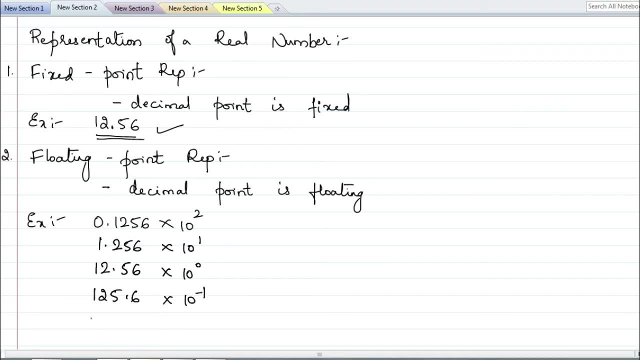 Or we can write 125.6 into 10 power minus 1.. Or 1.256 into 10 power minus 2.. So like this, various ways we can write, all these various formats of numbers represents the same value: 12.56.. 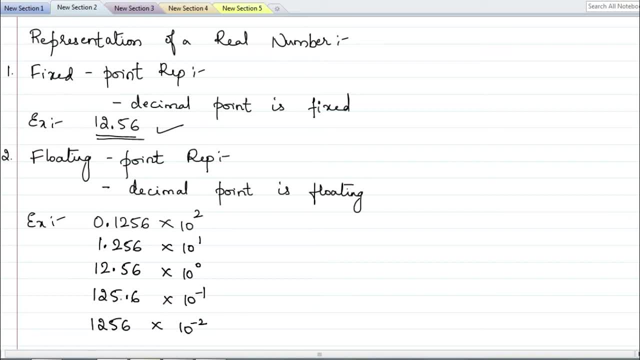 Here. if you observe, this decimal point is moving towards the right, Isn't it? So, since the decimal point moves towards to and fro, we call this as floating point numbers. We say the point is floating. Okay, that is the reason the name is coined this way. 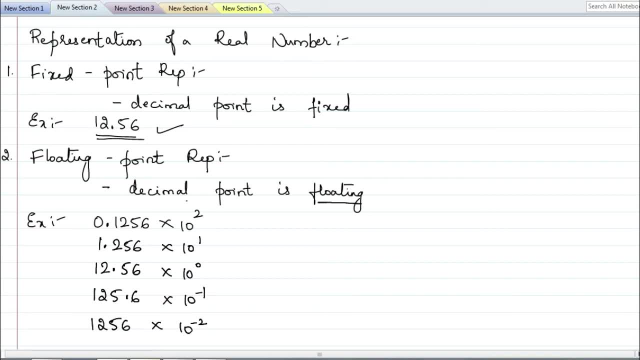 Now, if you have to understand when certain numbers are given, like this in a problem, you will have to make certain arrangements in order to solve it. So remember, if you have a decimal point, if it is moving towards the right, then decrease the power. 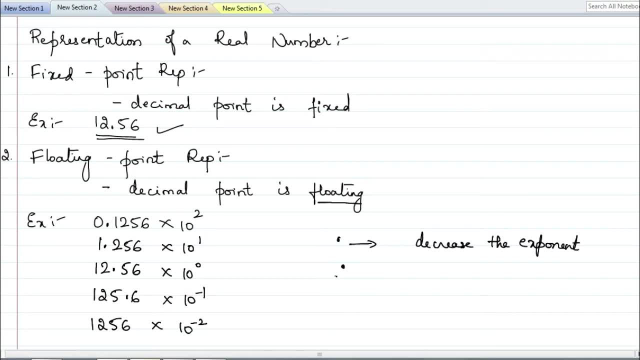 Okay, decrease the exponent. If the decimal point moves towards the left, then increase the exponent. Remember this: Say: if I have 123.5678 into 10 power minus 3.. So this is a number If I move the decimal point towards the right side. so I will move the decimal point from here to here. 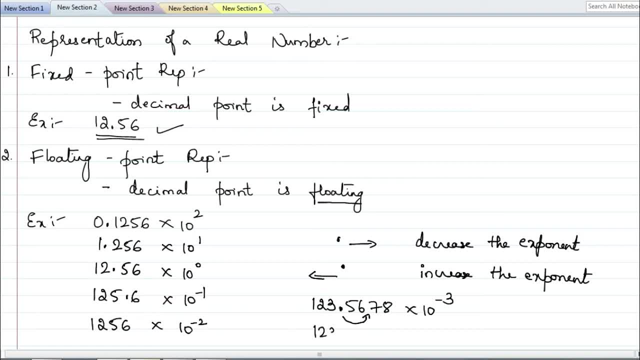 Okay, I will shift the point right side by two digits, So the number becomes 123.56.78 into 10 power. See if it is moving towards the right side. you are supposed to decrease the exponent Here, minus 3 is there. 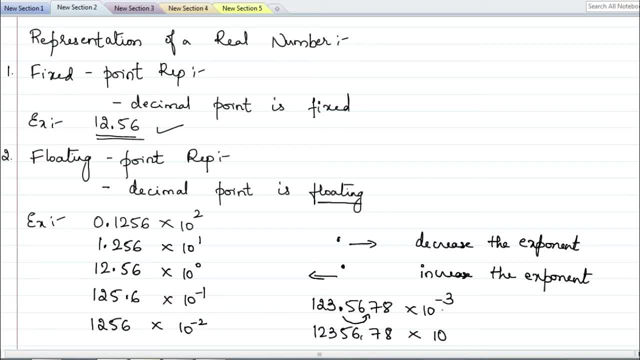 I will decrease 2 from the exponent because I am moving it. I am shifting it to the right side by two digits. So minus 3 minus 2 is minus 5.. Hope you understood I have shifted. I have shifted the decimal point to the right by two digits. 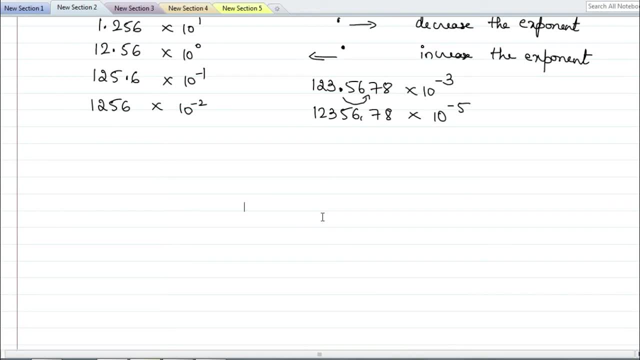 Therefore, I will decrease the exponent by value 2.. So if the same number instead of this, if I shift the decimal point towards the left side by one digit, So the number becomes 12.35678.. Right, So I have shifted the decimal point to the left by one digit. 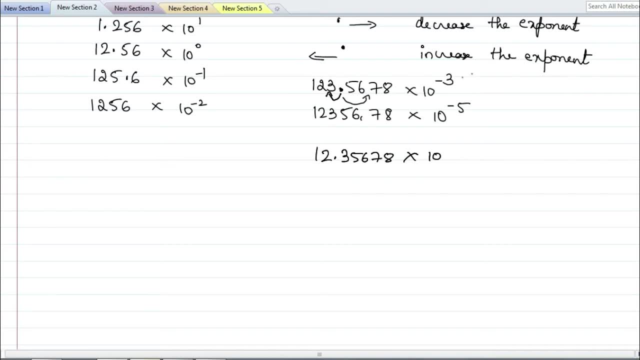 So I need to increase the exponent by 1.. So minus 3.. Plus 1 is minus 2.. Both represents the same value. Shift the decimal point to the right. It means you have to decrease the power. Shift decimal point to the left. 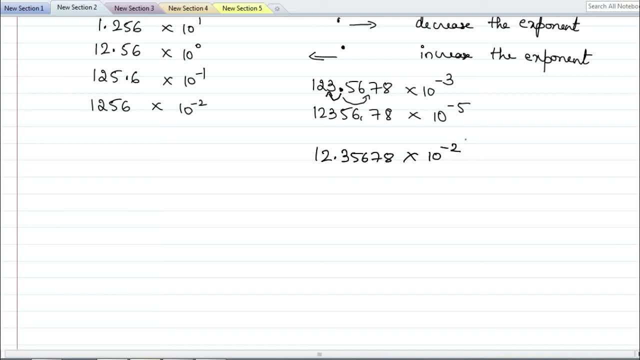 Then you have to increase the power. How much decreasing or increasing you have to make, It is equal to the number of digits you shift. Okay, So that is how you change the given number according to your requirement to solve a problem. Now, when you have a number like this, this entire number. 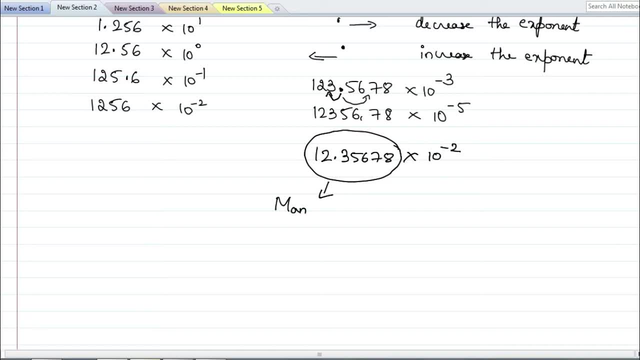 This is called as the mantissa. This 10 is your base And this power is called as the exponent. Okay, So this is a floating point number representation. You have a mantissa base and exponent. This is one way of representing a number. 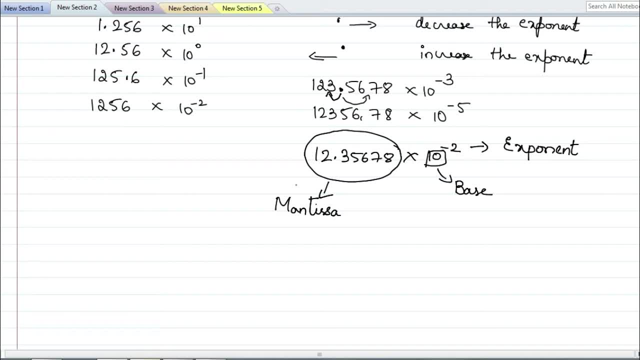 You can also represent the number using E. So this is a floating point number representation. So this is a floating point number representation. So this same number, you can write it as 12.35678, whatever E minus 2.. 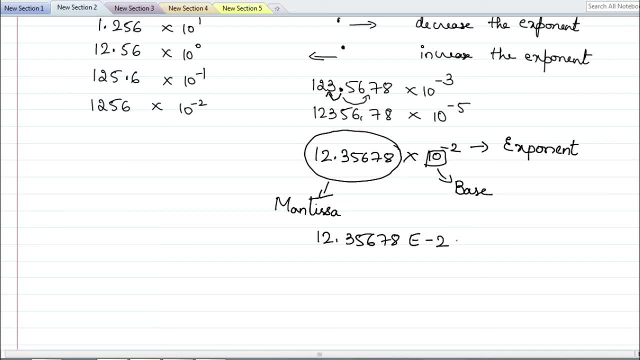 So this E represents into 10 power. For positive power you can just write E plus 2 or just E2.. So this is how you represent a floating point number. Next we will see what is a normalized floating point number. 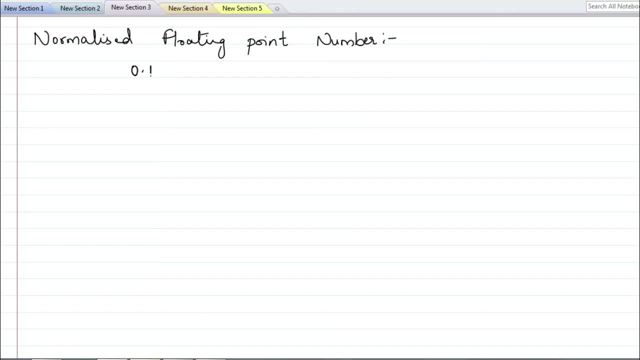 Normalized floating point number is a number in which the mantissa is greater than or equal to the number of digits And it is less than 1.. This is the definition of a normalized floating point number. So what is the meaning of this definition? 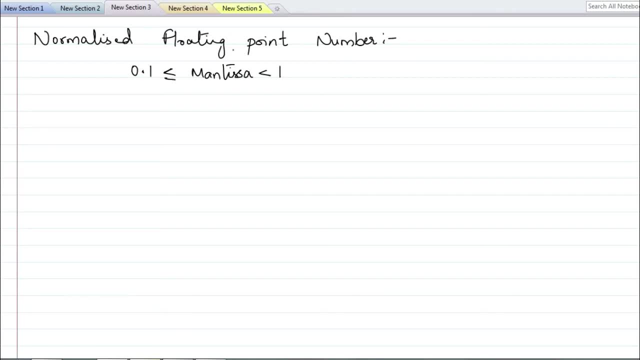 In a given decimal number. before decimal point, you should not have any non-zero number. Before decimal point, it should always be a 0.. Immediately after decimal point, you should not have a 0. That is the definition. That is the meaning of this definition. 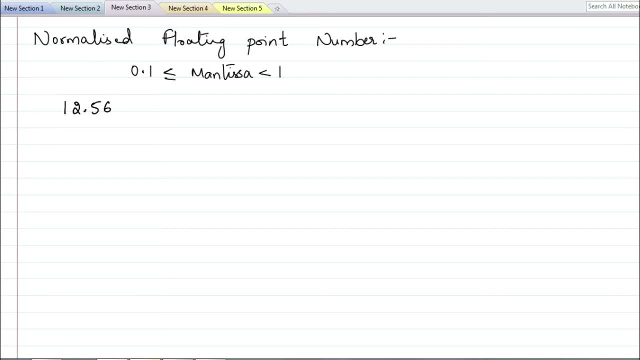 So 12.56 I had given as example. So I have to write it as 0.1256.. Before decimal point it is 0.. Immediately after decimal point it is non-zero. So this is normalized representation of a floating point number. 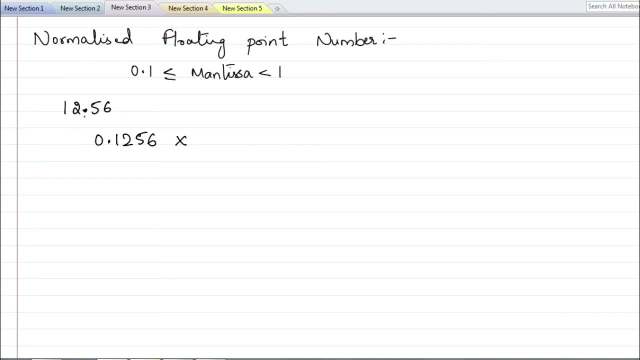 And here we have done the modification So the decimal point is shifted to the left by 2 digits. Therefore I need to increase, So I have to increase the power by 2 digits. So when there is no power it means it is 10 power 0.. 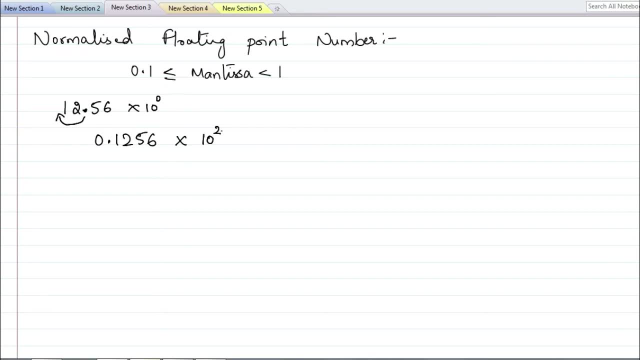 So I have to increase the power by 2 digits. This is normalized representation of a floating point number. So I will show you one more example. So let me take 123.48 into 10 power minus 6.. Suppose this is a number. 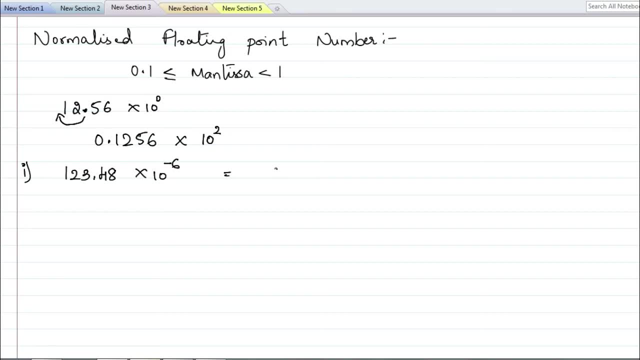 What is a normalized floating point representation of this? I have to write 0.12348.. Because, as I told you before point, you should not have any numbers Immediately after decimal point. you cannot have zeros. So it is 0 immediately after decimal point. 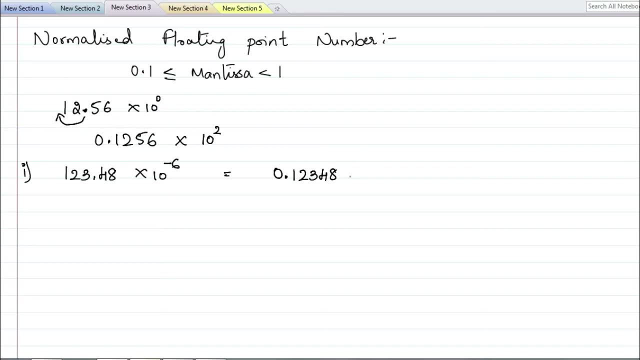 After few digits you can have 0. So 0.12348 into 10 power. Now what have I done? I have shifted the decimal point to the left side, So I need to increase the power By how many digits I have shifted? 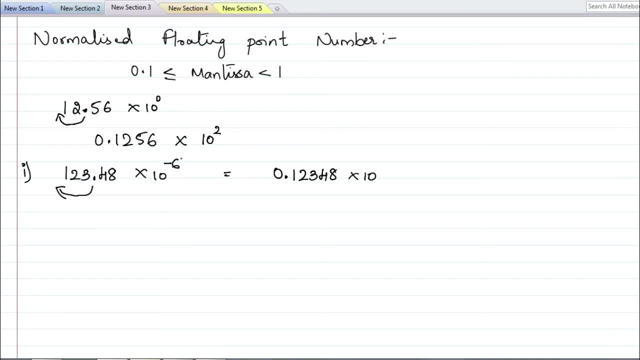 I have shifted it by 3 digits, So I need to increase the power by 3.. 3 means minus 6 plus 3. So it is going to be 0.00246 into 10 power minus 3.. 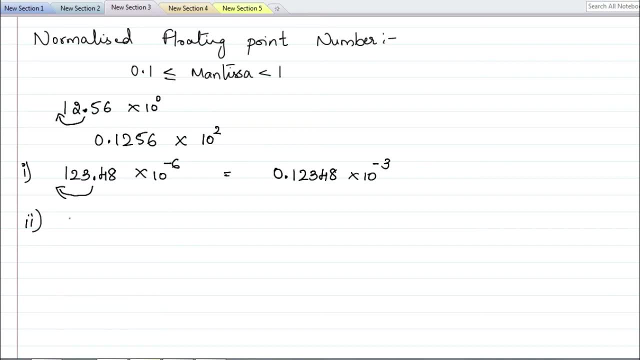 Okay, One more example. I will write 0.00246 into 10 power minus 3.. Okay, This is another example. Here again, this is not normalized floating point number, Because before decimal there is 0. But immediately after decimal it should not contain 0.. 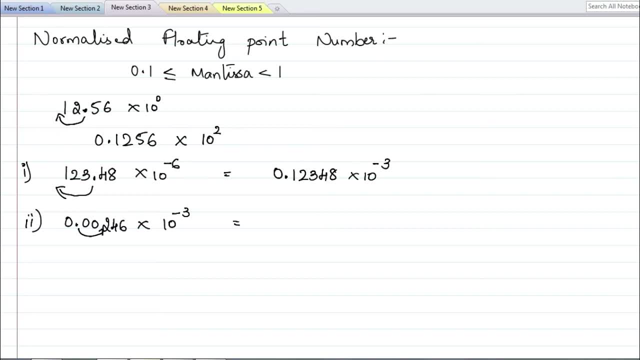 But it contains 2 zeros. So I have to shift decimal point to this position. So it becomes 0.246 into 10 power. Since I have shifted the decimal point to the right, the value decreases. By how many digits have I shifted? 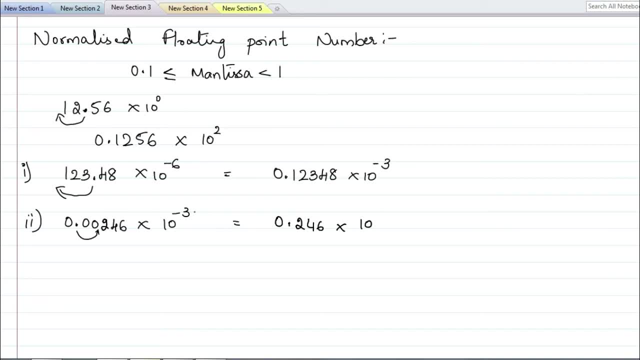 I have shifted by 2 digits, So I have to reduce 2.. So minus 3 minus 2 is minus 5.. Okay, This is converting a given number to normalized floating point number. Almost for all the calculations we will be considering normalized floating point number only. 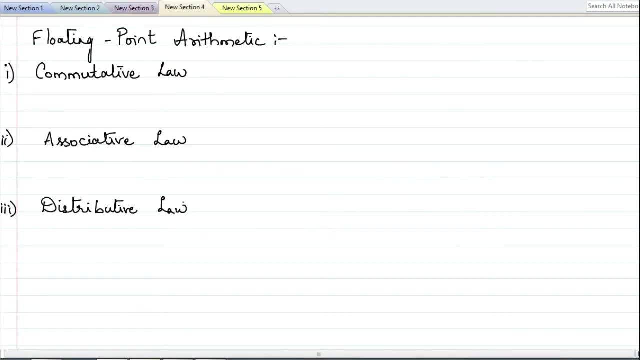 So the next topic is Floating point arithmetic. Here we will be covering 3 laws: Commutative law, associative law and distributive law. I am sure all of you would have studied these laws in your high school itself, So we will just quickly see what is a commutative law. 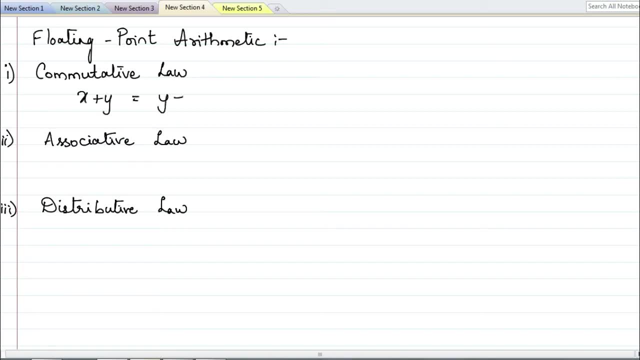 x plus y equals to y plus x, So I will be covering only laws of addition. The same rules is applicable for laws of multiplication also. That is, x into y equals to y into x will also be the other form of commutative. 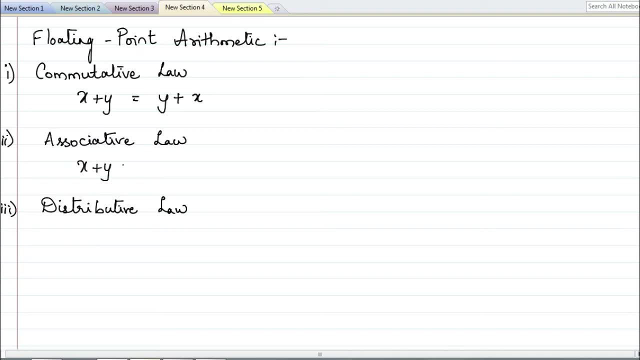 Next is associative law, That is, x plus y plus z. When we have 3 variables, then how do we associate them, Means how do we group them? So x plus y plus z will be equal to x plus y plus z. 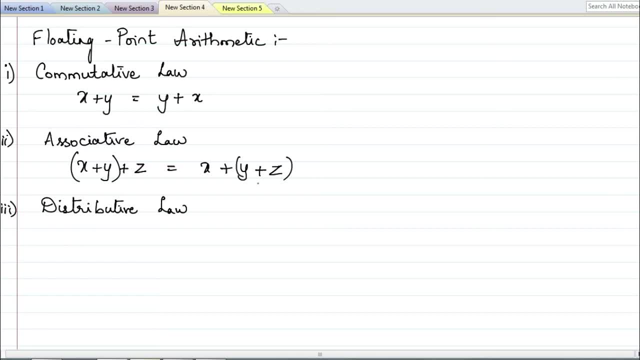 This is associative law of addition. The same thing is applicable for multiplication also. x, y into z is equal to x into y z. That is associative law of multiplication. Next is distributive law. Distributive law is x into y plus z is equal to x y plus x z. 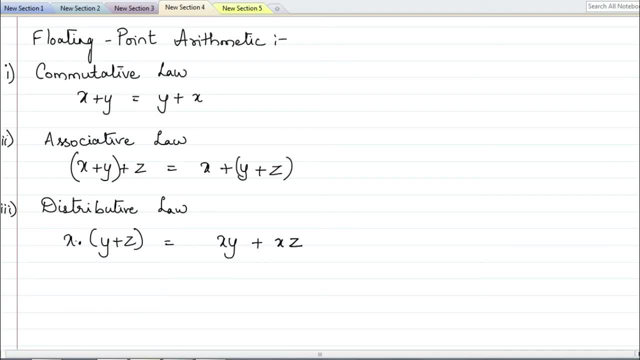 This is distribution of multiplication over addition. So these are the common laws that governs all the arithmetic operations of the numbers. Now, floating point arithmetic satisfies commutative law, Means when you have 2 floatings. So floating point numbers x and y. 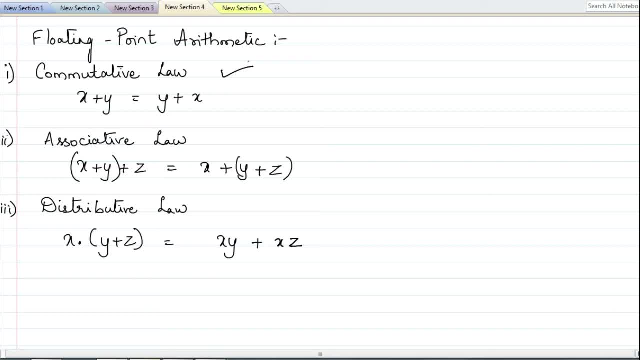 Whether you add x plus y or y plus x, the answer is going to be same, Whereas it does not satisfy associative law and distributive law. So when you first add x plus y and then add z, or if you add y plus z and then add x to it, 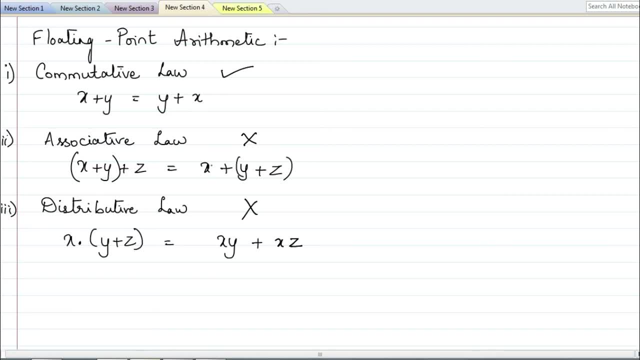 So the answer: the LHs and RHs may not be equal. Sometimes it might be equal, but sometimes it might not be equal. So the questions under this category will be: They will give You certain variables with some values. They will give you a formula also. 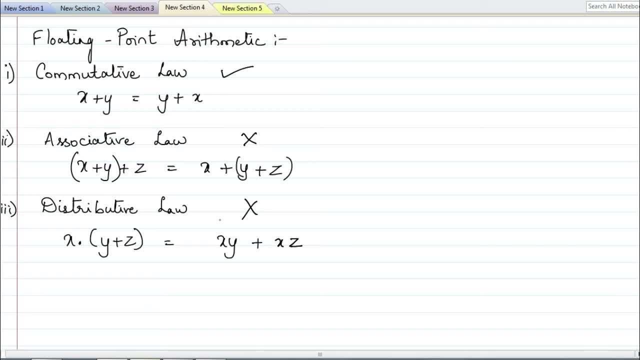 Basically it is going to be associative law or distributive law only. They might not give you commutative law. They will give you associative or distributive law. They will ask you to verify it. Most of the times, LHs will not be equal to RHs. 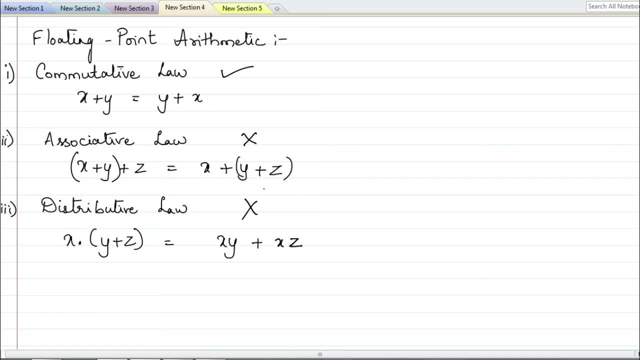 You have to find the value of LHs, Find the value of RHs and then show that they are not equal, So associative and distributive laws are not equal in this case. Now, Before we see a problem under this category, We will first see. there is one approximation technique that you need to use. 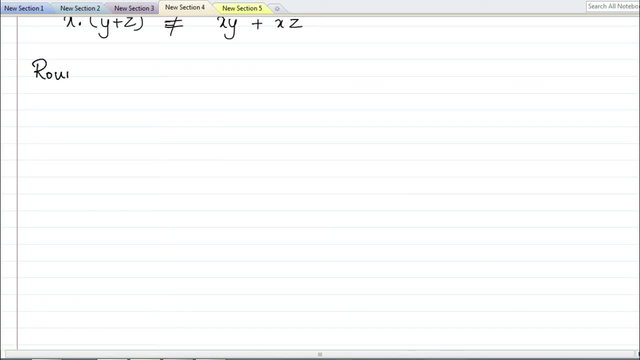 So how do we approximate? We have two methods: rounding and chopping. So I will tell you what is rounding. Chopping is just chopping of the numbers, Okay, So we will see what is rounding. So we have all done approximation. 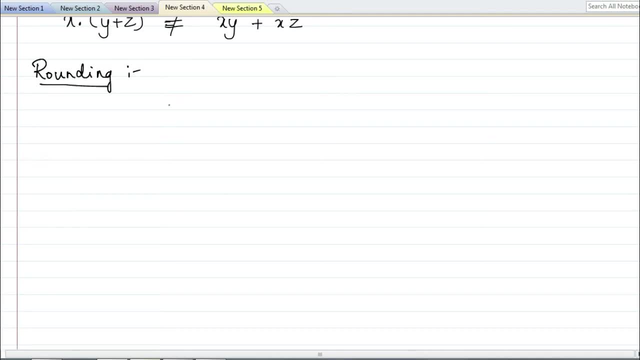 Right. So what is? how do we do approximation? Suppose we have a number like this: 0.4586.. So if I tell you approximate it to three digits, It means you will consider only the first three digits after decimal point. 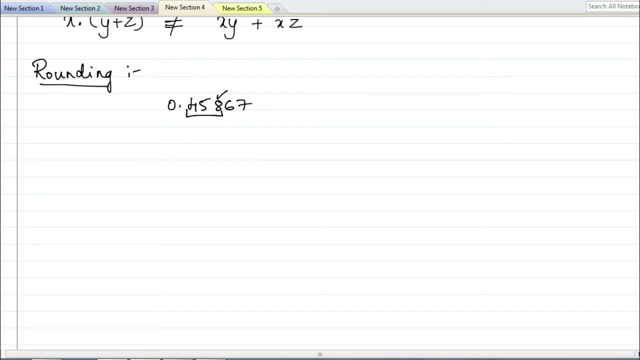 So when you are considering approximation, You will modify this third digit based on the value of the fourth digit Right. So that is how we do the approximation. How do we do? usually? If it is less than 5, we keep the number as it is. 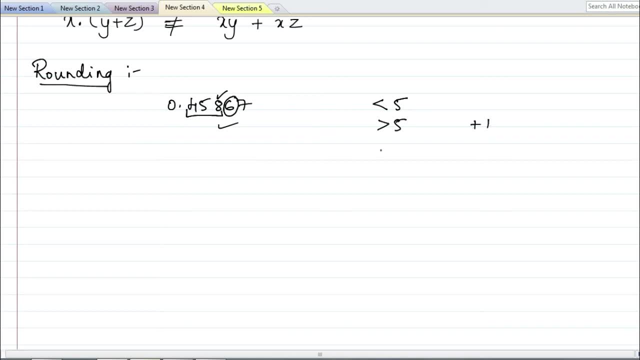 If it is greater than 5, we increase 1.. What if it is greater than 5?? What if it is equal to 5?? This is one additional rule that is included under floating point arithmetic. When we do three digit approximation, then third digit is approximated based on value of the fourth digit. 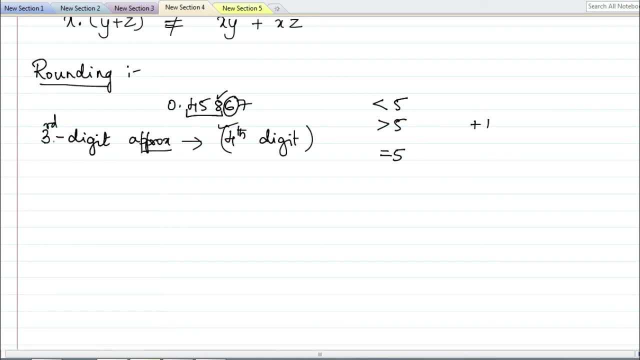 If fourth digit is less than 5, then third digit remains same. If fourth digit is greater than 5, third digit is increased by 1.. So this, both things. all of us know that is how you have been doing the approximation. Suppose fourth digit. 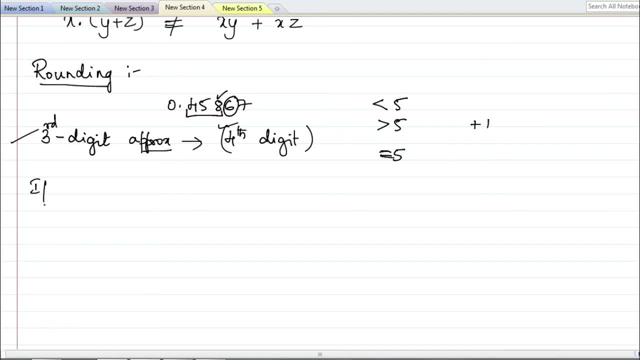 Is equal to 5.. So if fourth digit, or in this case n plus 1th digit, If we want n digit approximation, we need to check what is n plus 1th digit. If n plus 1th digit is equal to 5, then if third digit is an even number, then do not change it. 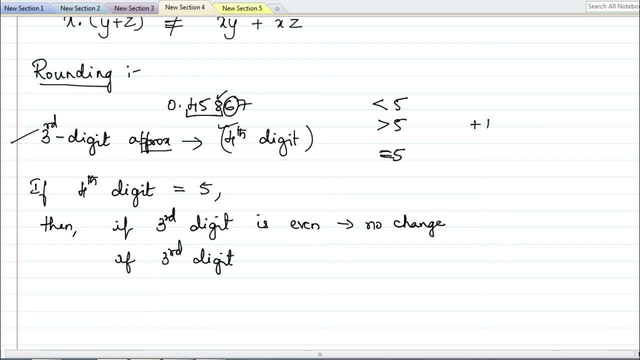 No change. If third digit is an odd number, then increase 1.. Add 1 to it, Increase by 1.. So let me take some examples. Suppose you have a number, the same number, I will take 0.45867.. 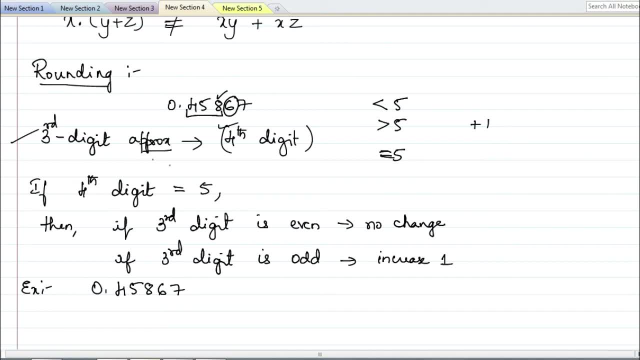 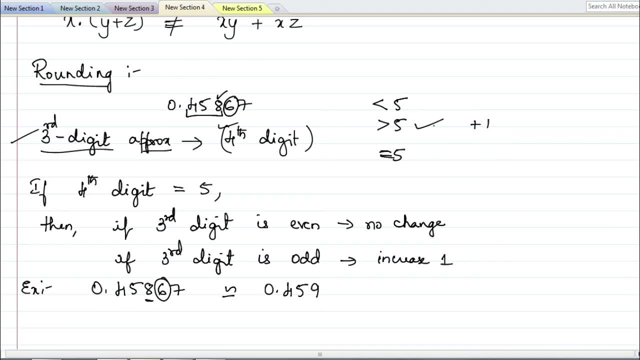 0.459.. 4th digit is greater than 5, I will approximate 8 to 9.. Suppose I have 0.45827, then I will consider third digit as it is, because 4th digit is less than 5.. 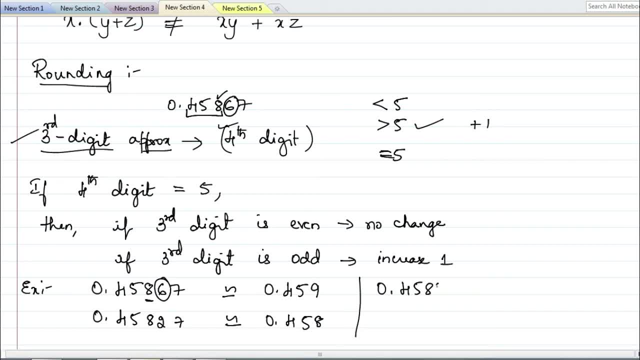 Suppose I have 0.45857, so I need three digit arithmetic. 4th digit is 8 to 9.. Suppose I have 0.45827, so I need three digit arithmetic. 4th digit is exactly equal to 5. in that case, check the third digit. if third digit is an even number, write it as it is. if third digit is an odd number, I will take 45757. okay, so I need three digit arithmetic. 4th digit is exactly equal to 5. in this case, see what is third digit. it is an odd number, so increase by 1 so it becomes 0.458. okay, so this is approximations technique that you need to know. 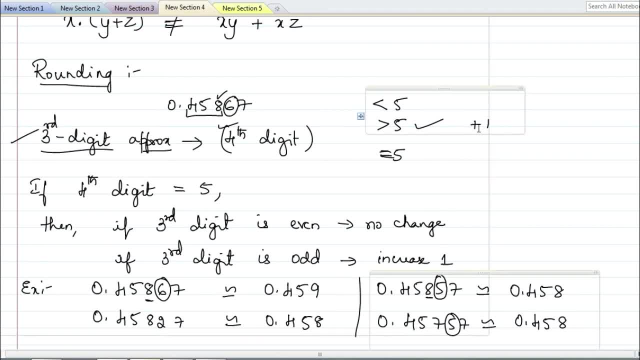 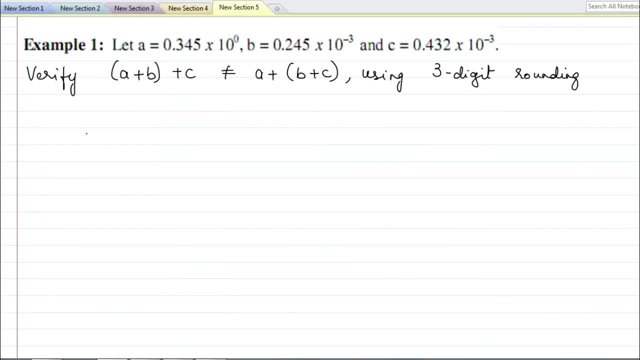 you need to apply and based on this approximation only, you will have to solve the questions. let's see one quick example. so this is an example question. here we need to verify the distributive law using three digit rounding. here, before we start solving, first thing you need to observe is make sure that all exponents are equal. okay, so make all exponents equal. if they are not equal- mostly in such cases- 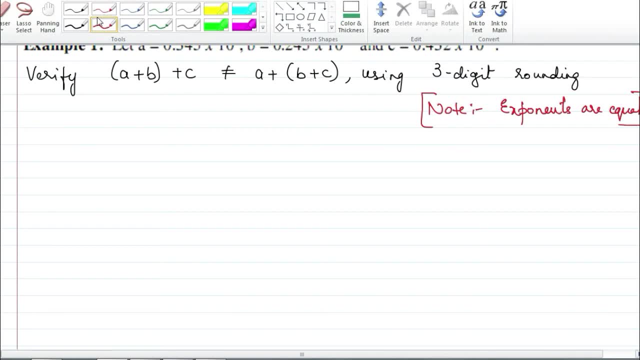 definitely one of the exponent at least will not be equal, so let's make them equal. see here how to make it equal: the one that is lesser that you increase to make it same as the exponent which is greater. see here: 10 power- 0 is there. this is 10 power minus 3. here we have minus 3. 0 is greater than minus 3, so we need to add plus 3 here to make it same as this exponent understood. 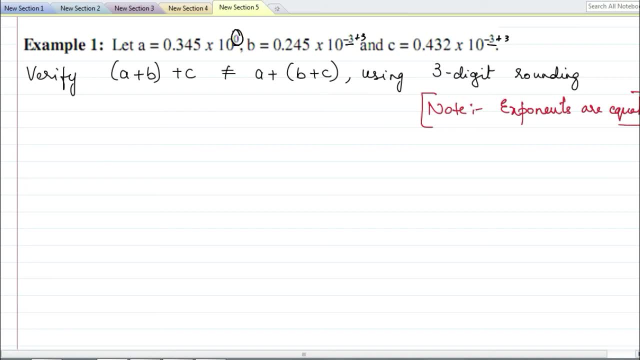 so, first thing, what we need to do is make it same all the exponents. you need to make it same. to do that, don't reduce the power of a bigger exponent. instead increase the power of smaller exponents. so minus 3 is smaller. here I'm increasing, I'm adding plus 3 to it so that it becomes a same as the higher exponent. when you're adding plus 3, it means you need to add three zeros after decimal point. okay, so now what are the values? a is 0.5. 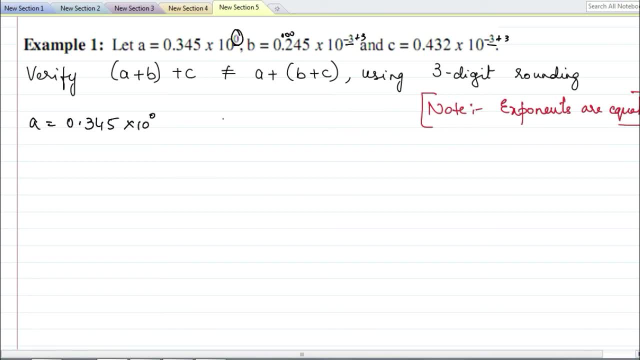 0.345 into 10 power 0 and b is 0.000245 into 10 power 0 and c is 0.000432 into 10 power 0. okay, now we will solve the given question. so what is lh is a plus b plus c. so first I'll find out what is a plus b. 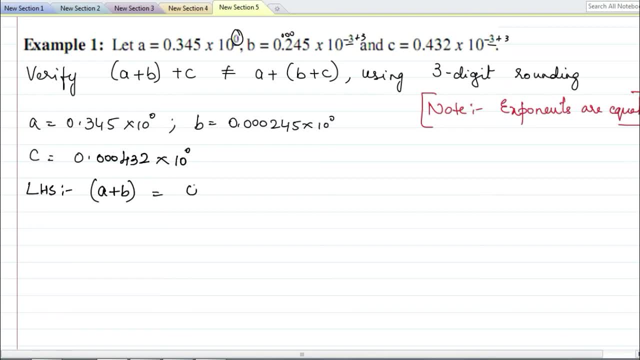 so when you are writing a plus b, I'm supposed to add 0.345 and 0.000245, and this is into 10 power 0 exponent. we can write it at once in the end, because anyways the exponents are equal. now add it, you'll get 0.345245 into 10 power 0. after each arithmetic operation we are supposed to do the rounding. 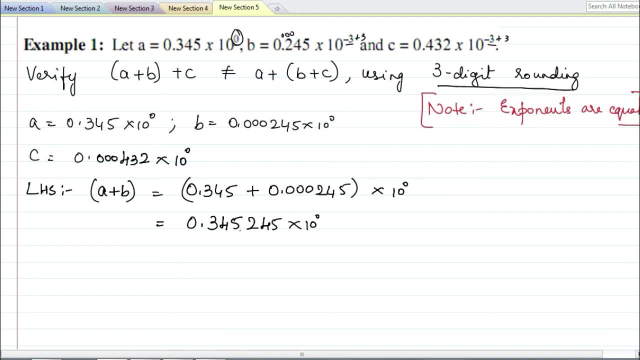 so since we are supposed to do three digit approximation, I will consider only first three digits and the third digit I'll approximate depending on the value of the fourth digit. so I will get 0.345 into 10 power 0, because fourth digit is 2. third digit remains as it is. now I'll add plus c to it: a plus b plus c. so what is a plus b, 0.345. 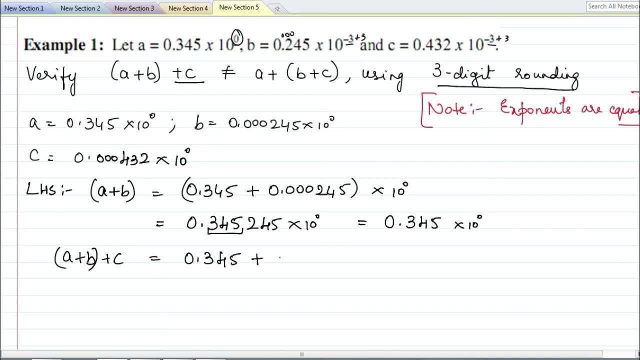 0.345.. plus what is c, 0.000432 into 10 power 0. now I'll add this: I'll get 0.345432 into 10 power 0. again, I'll make it approximate answer. I'll approximate it to three digits. we will get 0.345 into 10 power 0 this way. 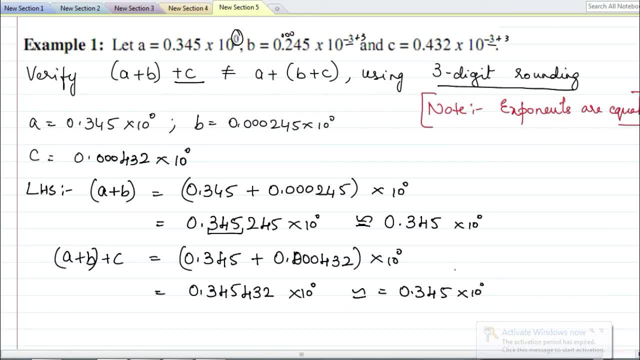 5. into 10. zero, because fourth digit is less than five. okay, so this is the answer for my LHS. this is the answer for LHS. now let's see what is the value for RHS. so RHS: first I have to do B plus C, then I need to add A to it, so I'll find out B plus C. 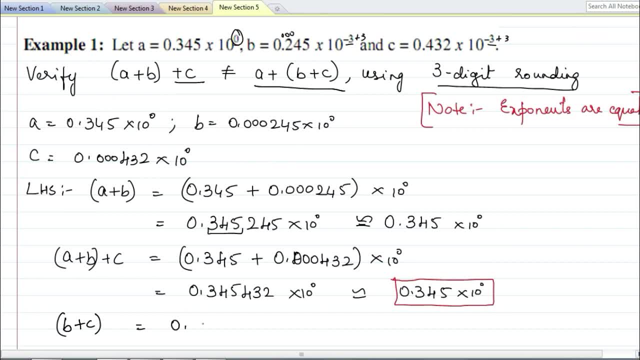 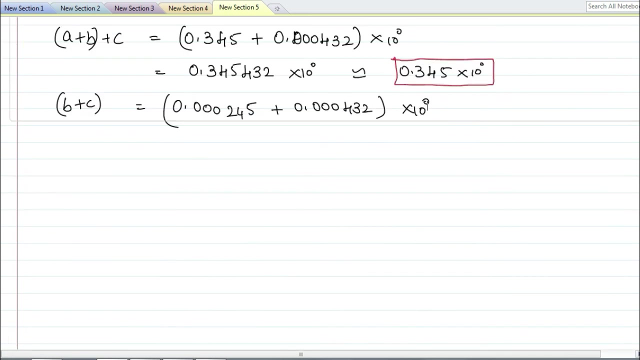 B plus C is 0.000245 plus 0.000432 into 10 power 0, you get 0.000677 into 10 power 0. since we have to use normalized floating point numbers, we need to write it as 0.677 into 10 power minus 3. so this is going to be the answer for. 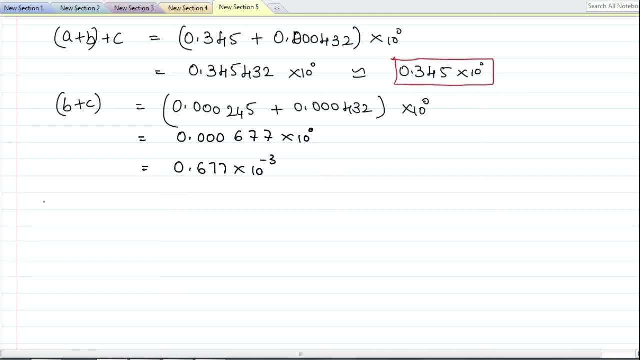 B plus C. next we need to add A to this. so when we add A, A is 0.345 plus this. I have to write it as per the standard form. I have this value. I'll write it as per the X by equating the exponent. 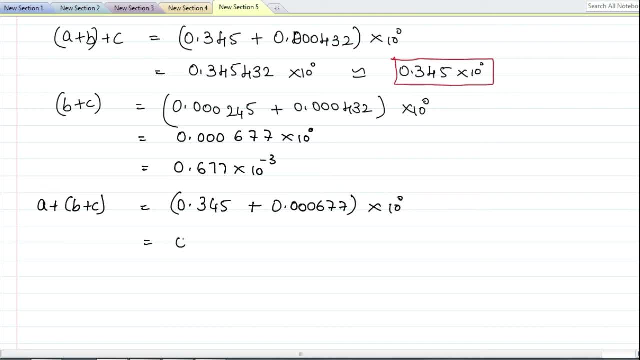 now I get 0.345677 into 10 power 0, so this I'll approximate it to three digits. I'll get 0.345677 into 10 power 0, so this I'll approximate it to three digits. I'll get 0.345677 into 10 power 0. 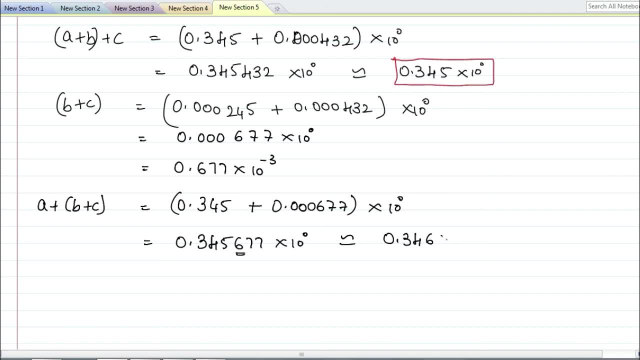 0.346, because fourth digit is greater than 5, into 10, part 0.. So now this is the answer for your RHS. okay, Clearly you can see LHS is not equal to RHS, okay, So therefore you can write LHS not. 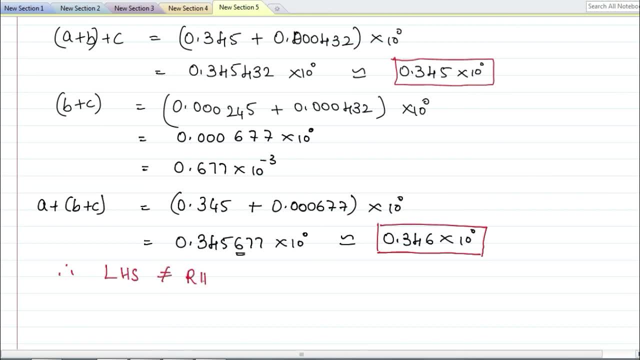 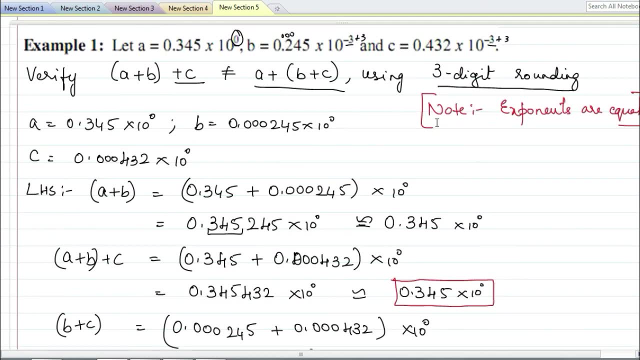 equal to RHS. therefore, given statement is proved okay. So this is how you need to solve. I will just repeat the steps quickly. So first step is: first you have to observe whether exponents are equal or not and make the exponents equal. How to make exponents equal: Lesser exponent should be. 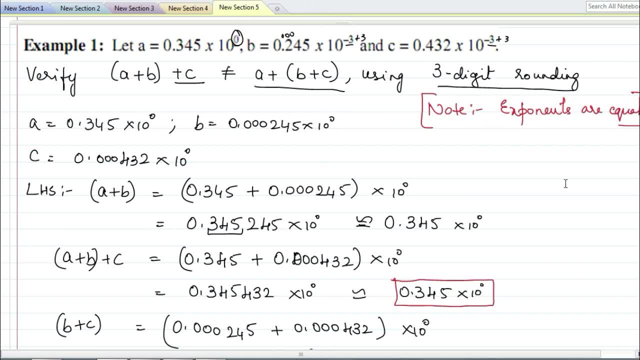 made equal to the greater exponent. So add some value to the lesser exponent so that it becomes equal. Now, however number you are adding to the power that many zeros you have to add after the decimal point. So this is one thing you need to know. Next is you have to find out what is the 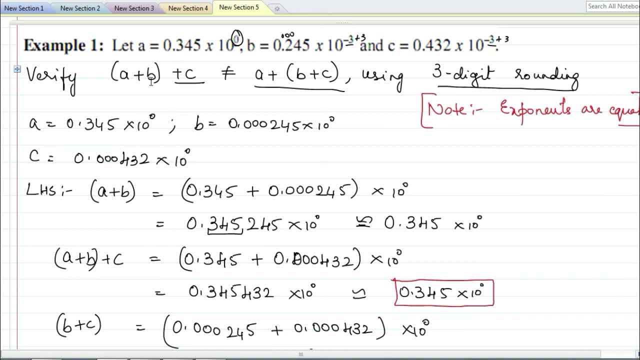 what is the value of LHS and RHS here? A and B, you are adding. so when you are adding A and B, A has a different power, B has a different power. hence you consider this way: okay: A and B values and then add C to it. after every step. take the approximated value as per three digit or two. 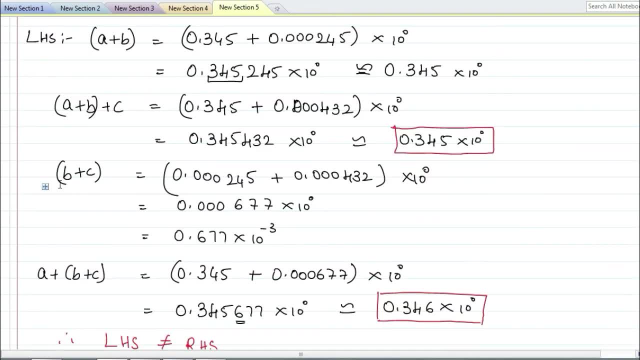 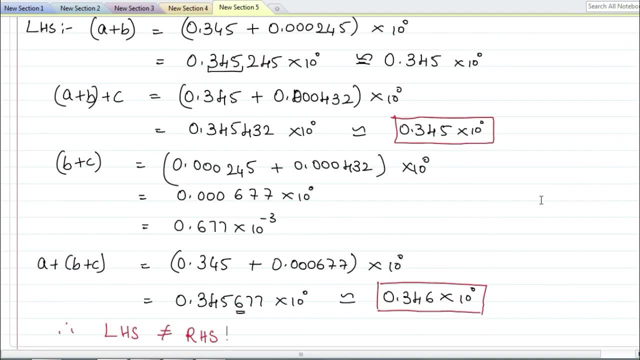 digit rounding whatever they have given. then take the RHS. in RHS you see B plus C is there and B plus C is has same exponent in the given question. so directly you can add: because the exponents are same, you need not have 10 power 0, you need to have exponents as same in this case. 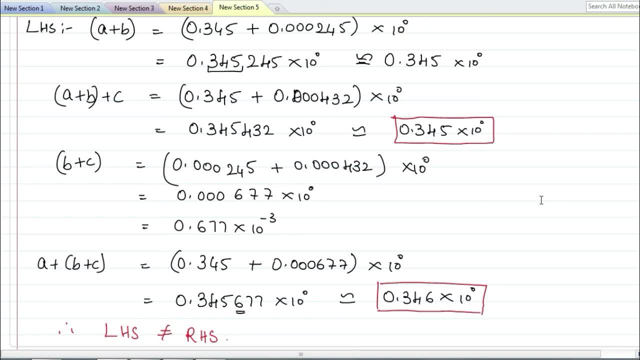 B and C has same exponents. so directly we can add without taking the zeros. you can directly add and get this answer. once you get this answer, next you need to add it with A. when you are adding it with A, make the exponent equal. so we are adding this: three zeros here and now.